and I would want to definitely hack into that. So what you want to do is you just want to rename it. Try not to make it too personally identifiable. Don't make it your name. if you can Just make it something that changes the name of the SSID and then allows you to know exactly what it is. 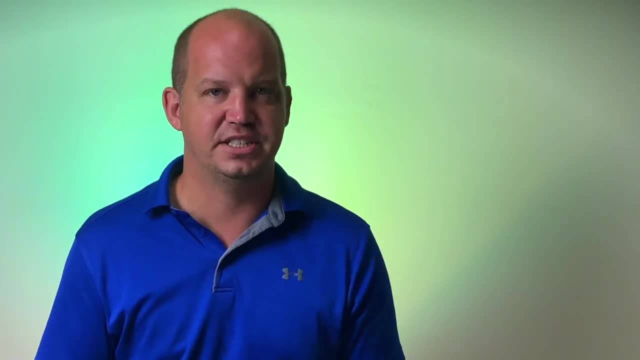 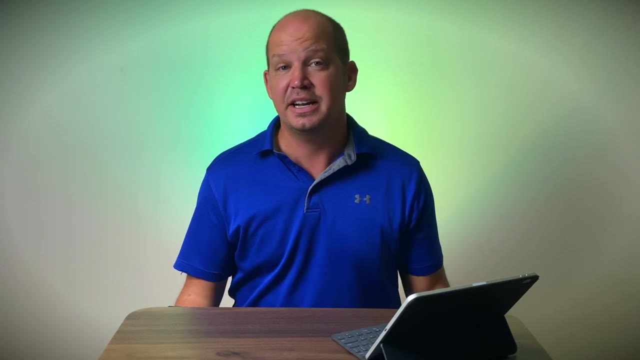 It's not going to make this super secure, but it is just a simple change that you can make While you're in there. the second thing that we want to do is we want to set up a new, more secure router. Obviously, your internet provider gave you a password and set up your Wi-Fi with password. 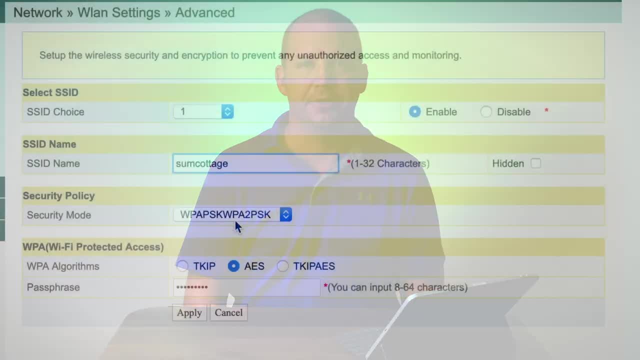 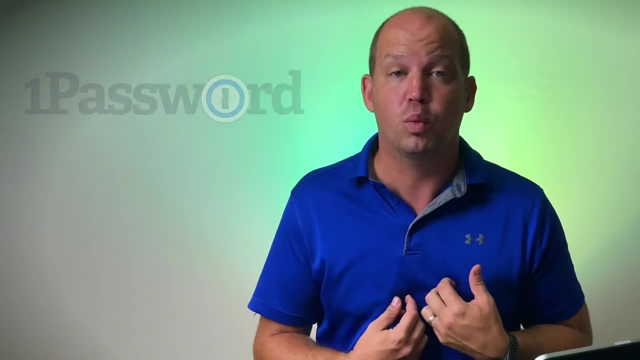 protection, but you want to do something that's maybe a little bit better, So you want to create a strong, unique password. I use a password generator and a password manager like 1Password to help me with stuff like this, And that's something you can consider as well. 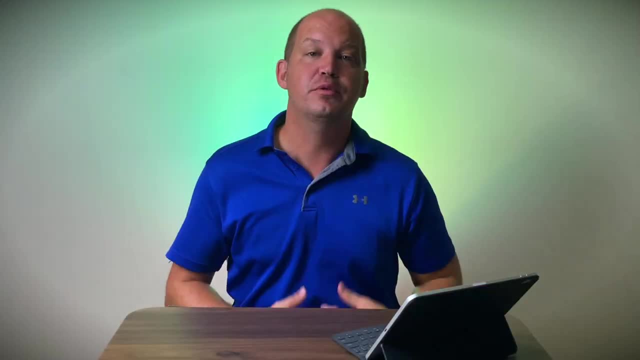 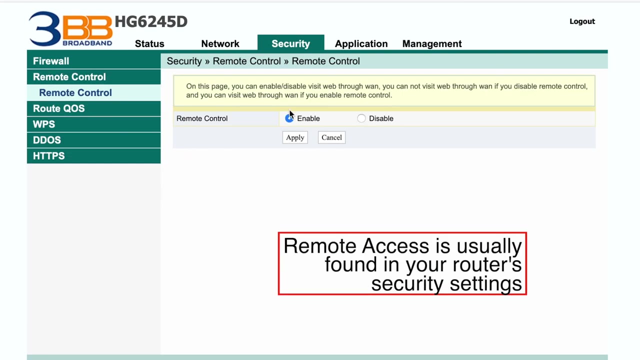 When you're in the settings for your router. another thing you want to look at is disabling remote access. There's very few times when you're going to want to have the ability to remotely access your router. What that means is if you're not physically present near the Wi-Fi router. 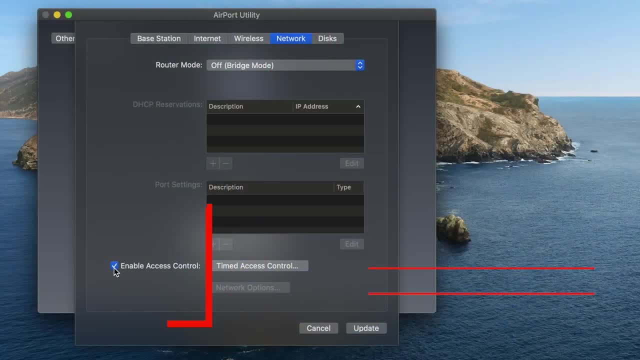 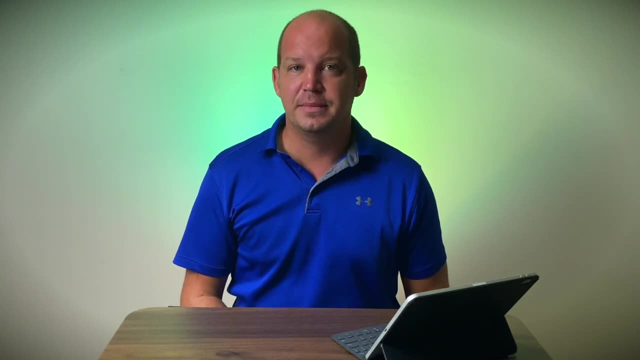 it's giving you the ability to basically dial in from another location And there's no reason that you're going to want to use that. for most people It's an advanced feature, so I recommend that you take and disable that feature if you can, If you have a lot of guests over. 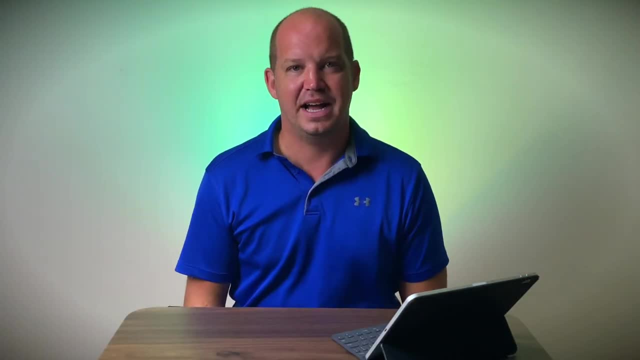 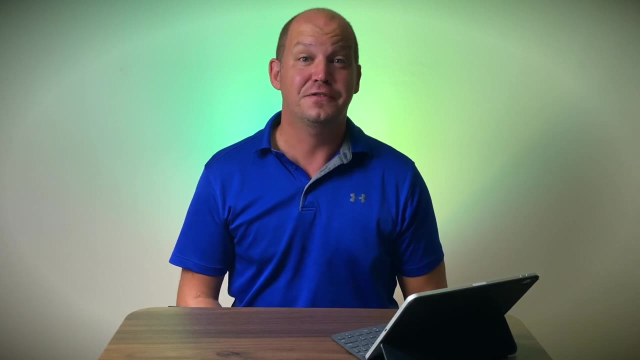 one of the things that happens is you tend to give out your Wi-Fi password And that Wi-Fi password gets stored in their devices for basically forever. If you were to look into your Wi-Fi settings, you'd find that you probably have quite a few networks that are remembered and saved. 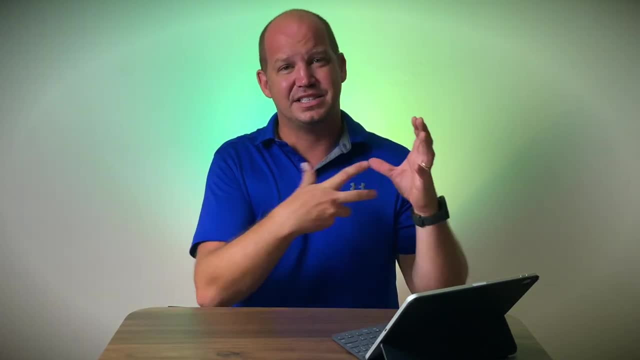 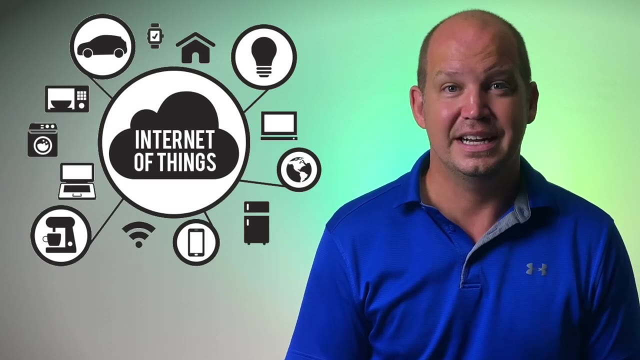 in your device. Now what that means is they also have access to your network. depending on how it's set up, That could even include your Internet of Things, devices like your Alexa or your Google Assistant, all of these things. So one of the things that I do that can be done. 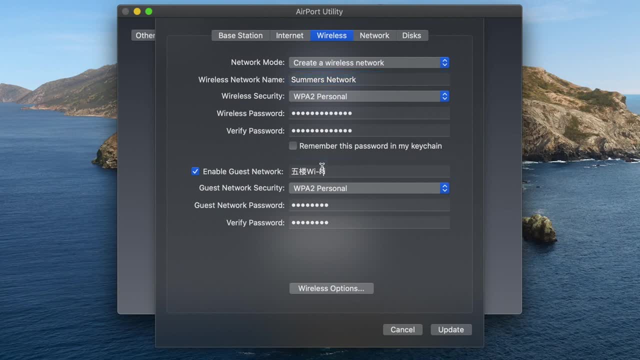 in a number of different ways, is setting up a separate Wi-Fi network for guests and other people. So I have a Wi-Fi network that's secured specifically for my family and our devices, And then I have a separate network that is for my Internet of Things. 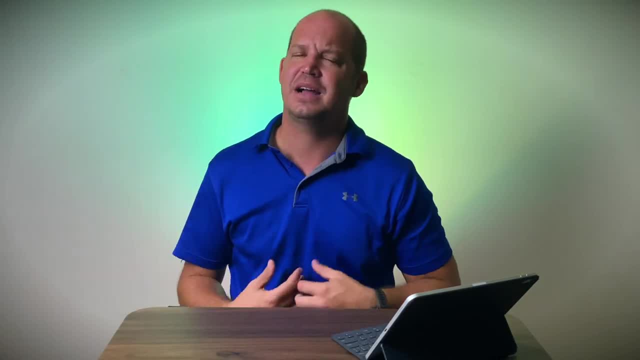 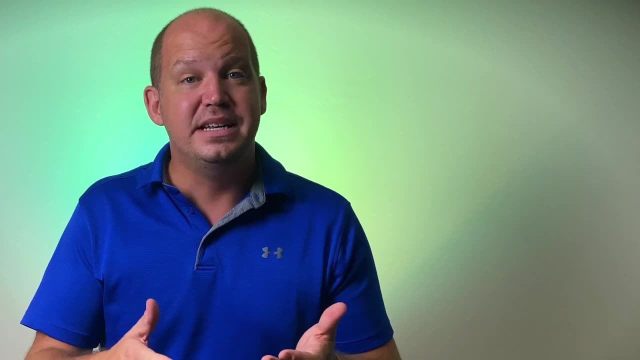 and for any guests that come in, So that when they ask for that password, I'm not giving away my secure password that I use for, you know, all of my Internet connection stuff. Now this can be done by having a separate router entirely, which takes a little bit of time to set up.